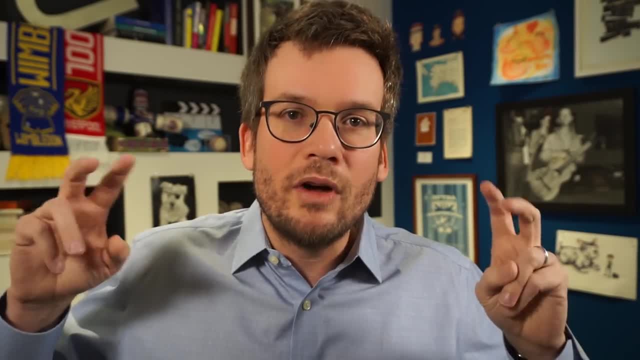 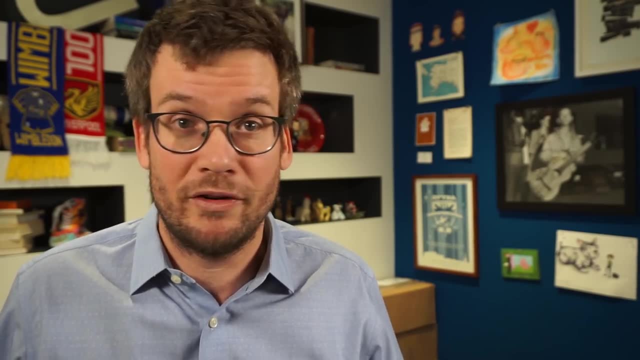 90% of the 95 million Americans not in the workforce say they do not want a job now. But the remaining 5 million people, of course, is a lot of people like it's 3% of the total US labor force. And some portion of declining labor participation is probably due to lack of job opportunities. People might have retired earlier than they otherwise would have because they lost a job or they might be in graduate school, but they could be tempted into the workforce for the right opportunity etc. 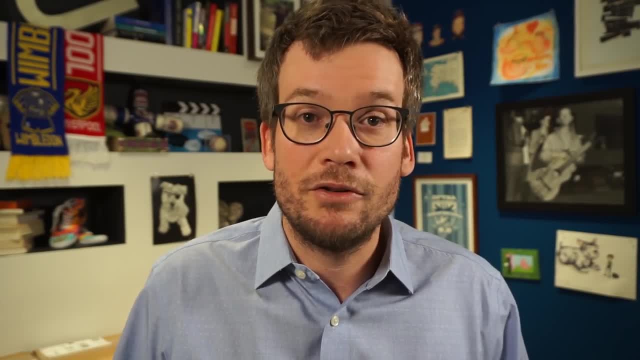 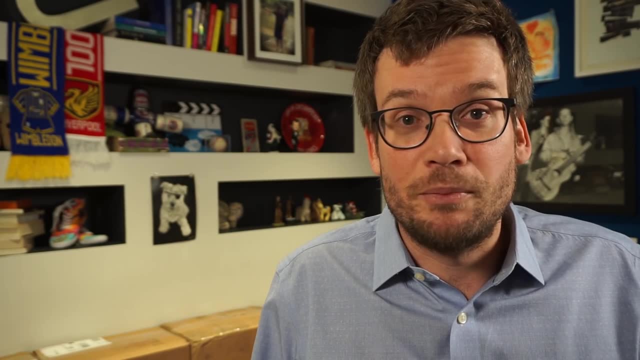 Now, smart people disagree about how much of the declining labor participation is attributable to the economy, but on its own, that statistic does not tell us much about unemployment. For one thing, the labor force participation rate will continue to decline as the population continues to age, whether the economy is good or bad, But also if you're going to claim that the real US unemployment rate is 38%, that means that back in 1967 it was 41% and that the lowest the US unemployment rate has ever been is 33% in 2000.. So let's move on to actual measures of unemployment. Every month, the US Census Bureau surveys 60,000 households to find out how many people are unemployed. Every month, the US Census Bureau surveys 60,000 households to find out how many people are unemployed. 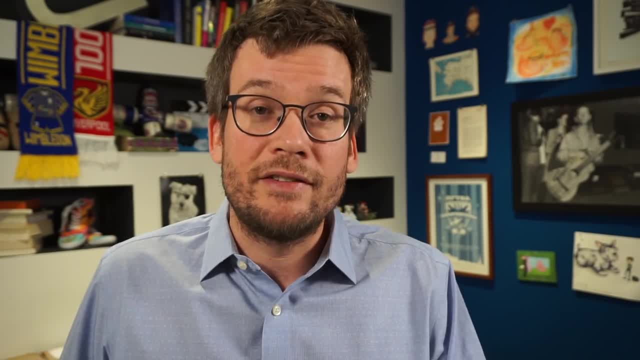 Every month, the US Census Bureau surveys 60,000 households to find out how many people are unemployed, And then on the first Friday of every month, they release six different unemployment rates, because nothing is ever easy, But for our purposes only four of them matter. 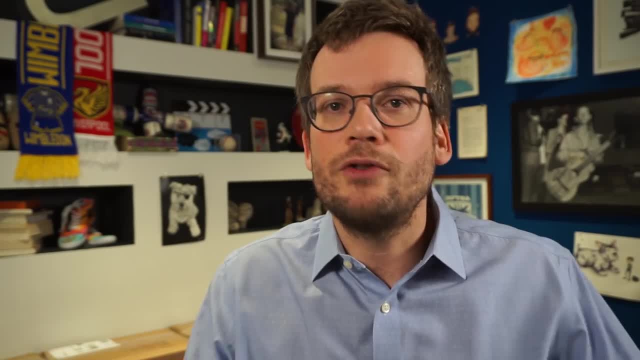 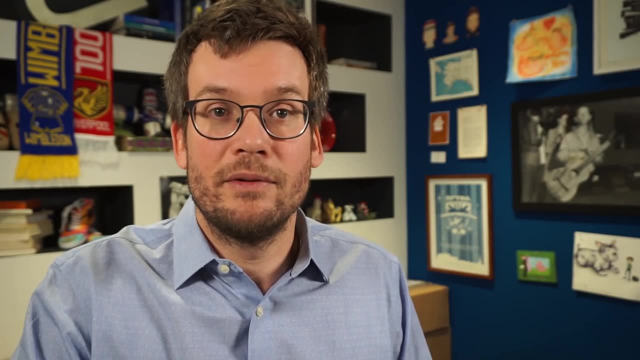 First you have U3, which is the official unemployment number. It includes all adult civilians who are without work and have looked for a job within the last four weeks. That's the number that's currently 4.7%. Then you have U4, which adds in so-called discouraged workers. 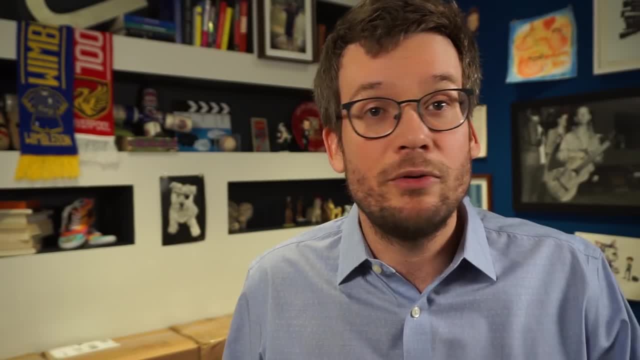 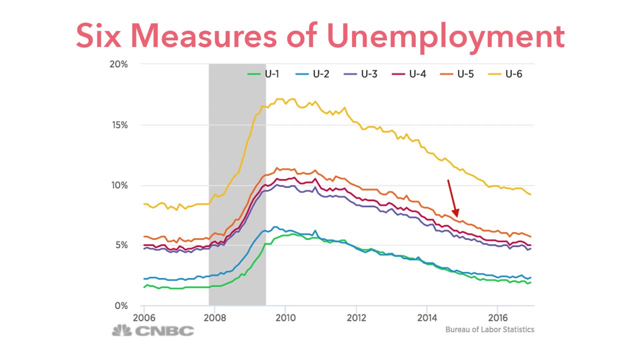 people who are without jobs but have stopped looking for work because they don't believe there are any jobs they can get. Adding them in raises the question: does the unemployment rate really matter? And then U5 adds in so-called marginally attached workers. 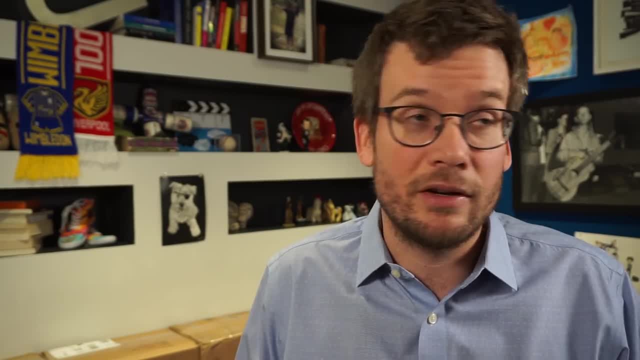 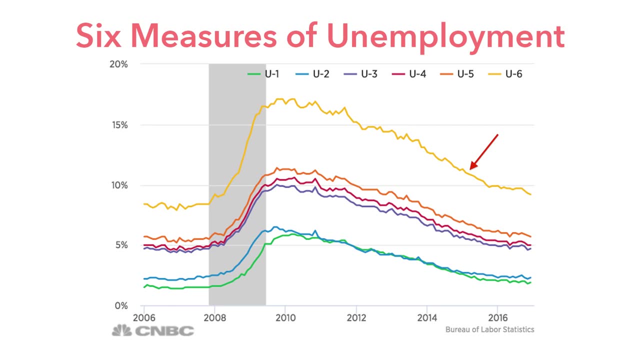 who are people who want to be in the workforce but haven't recently sought jobs because they're taking care of family responsibilities or taking classes, And they bring the unemployment rate up to 5.7%. And then, lastly, U6 includes people who work part-time but want to be working full-time. 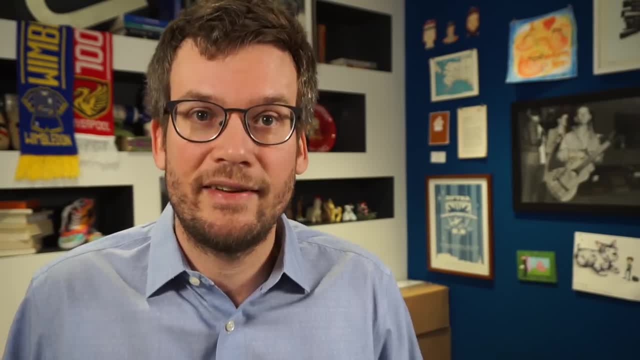 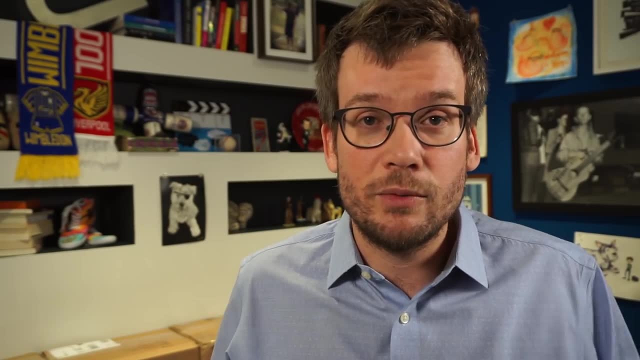 Including them brings the current unemployment rate to 9.2%. So which of these is the real unemployment rate? Well, it depends on what you're trying to measure. The U3 number is useful for one thing because it's closely aligned with the U4 number. It's also closely aligned with international standards, which allows us to compare our unemployment rate to that of other countries, Like in Brazil, a similar measure has the unemployment rate at 12%. In Germany, it's 4.1%. In Spain, it's 19%. 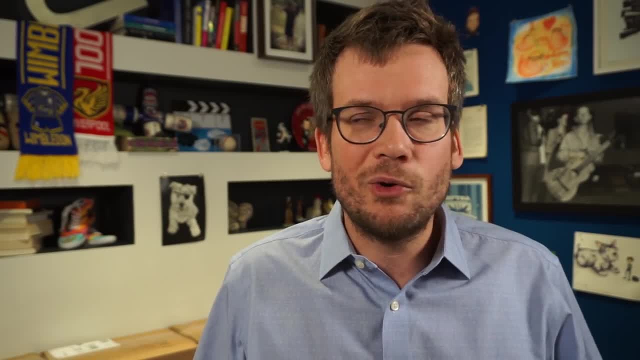 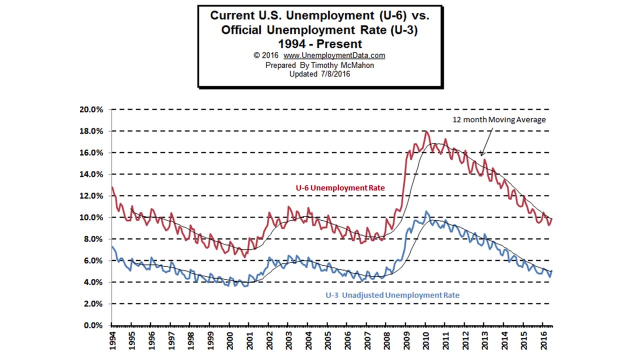 But the U6 number is also useful because it helps us to understand how much so-called slack there is in the labor market, That is, how much room there is for job growth. As you can see, U3 and U6 basically track together, but there are slight differences.